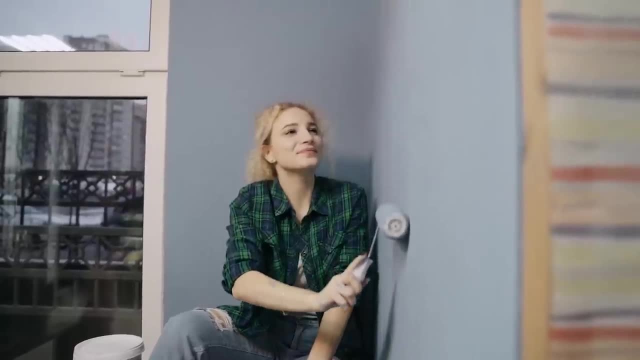 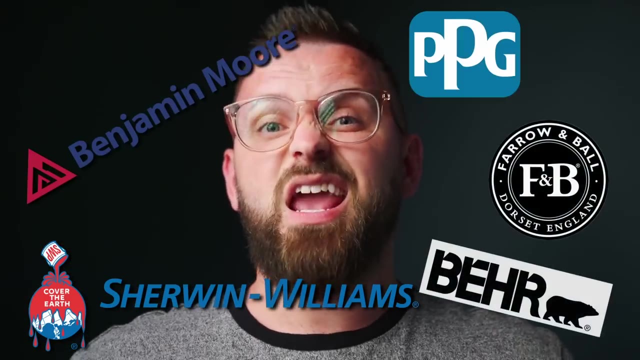 we do several videos a week all about painting and decorating. It's kind of our thing. Today's colors will be by Sherwin-Williams, But realistically you can have these paint colors made in any major paint products. They would just need to be custom color matched, which is also. 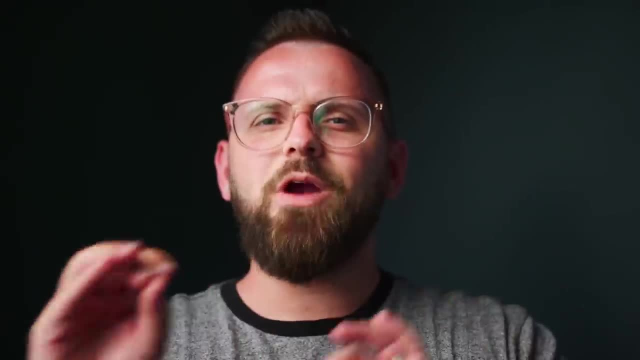 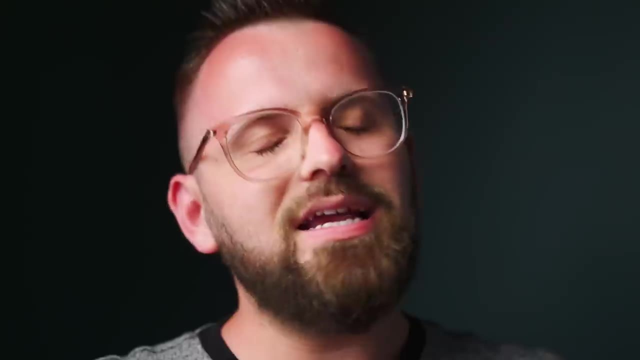 something I've experienced doing. That's enough humble bragging for me. Let's get right into these colors. And the first little grouping of paint colors are white paint colors, But more specifically off-white. I did not include the mega bright, high reflective white by Sherwin-Williams on this list. 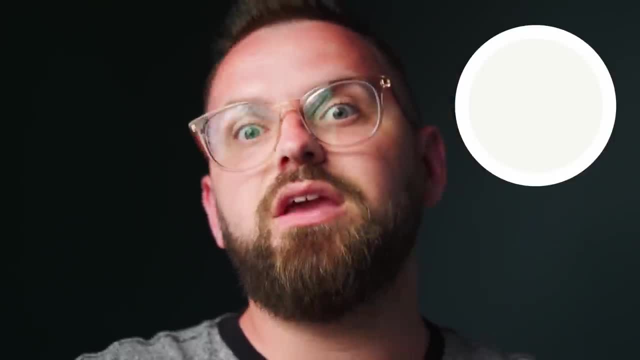 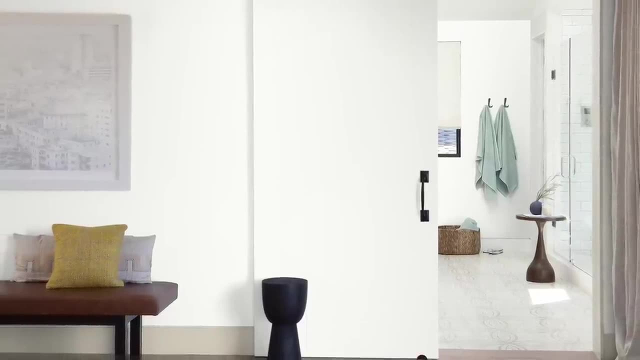 because I don't necessarily see it as a practical choice to paint your whole house with. That is one of the brightest white paint colors I've ever seen, which sounds good in theory if you want something nice and clean, But in practicality you won't be able to keep your walls clean because 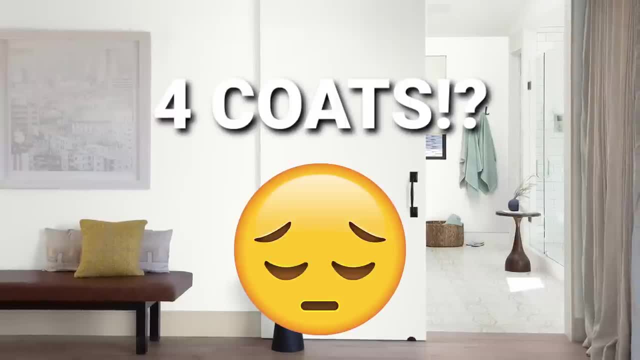 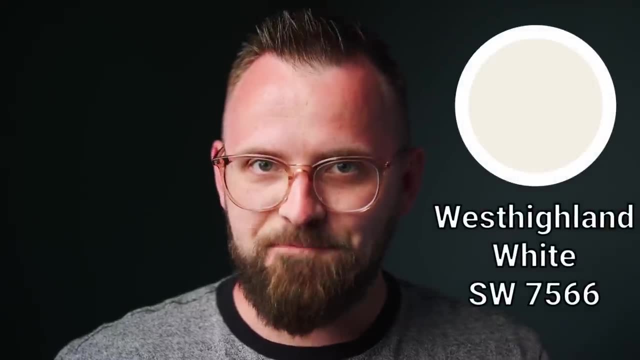 it's so bright and vibrant And it can also take four coats to cover properly, So not really an option for me. The first official entry on this list is called West Highland White And it really suits a number of different design styles pretty well. 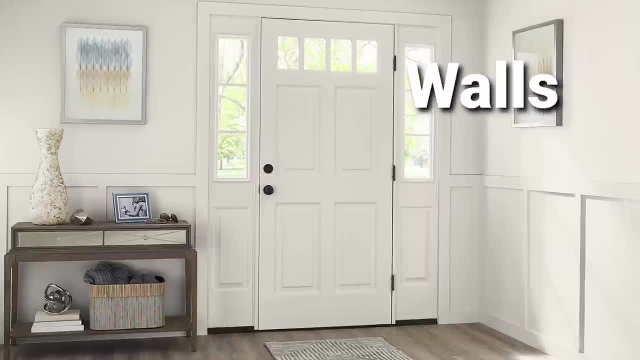 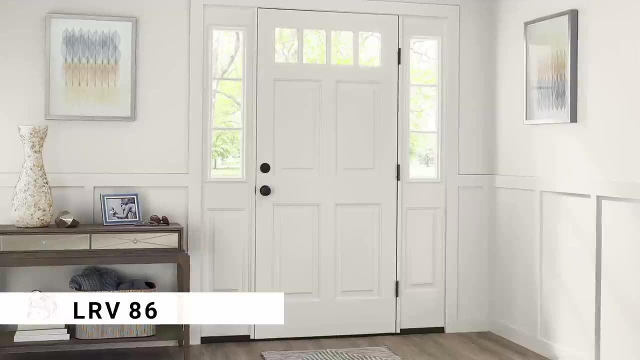 I would say it's light enough that you could theoretically use it on your walls, your trim and baseboards, even your ceilings, if you really wanted to. In fact, that's my favorite implementation of this color is enveloping the whole space in it, Sometimes when you have several. 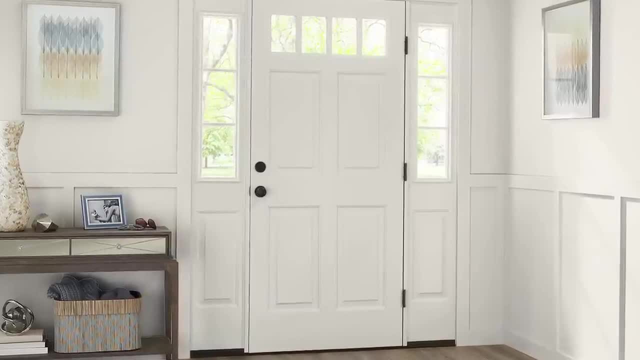 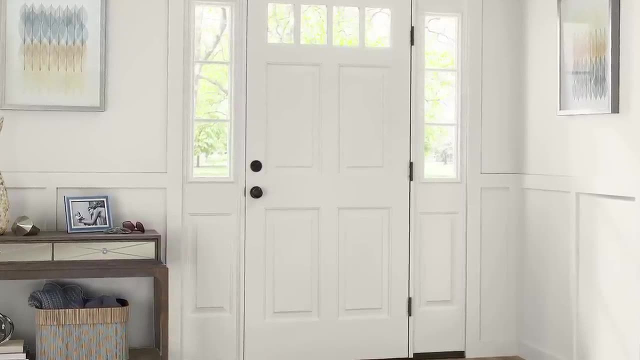 competing off-whites next to one another. it could clutter the whole design. So when you have the chance to simplify And you just paint everything one color, I think that's always a good option If you're not ready to have a slightly warmer. 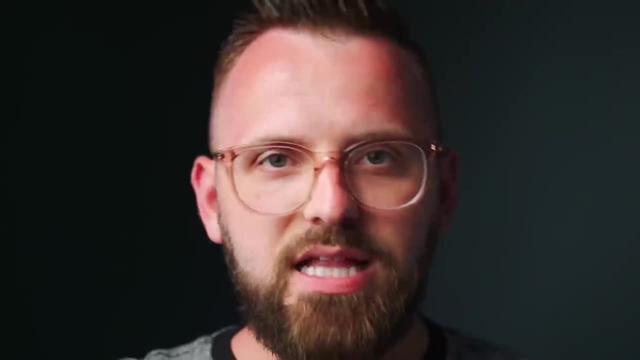 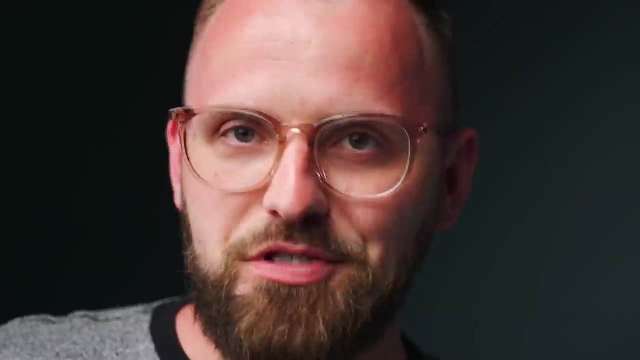 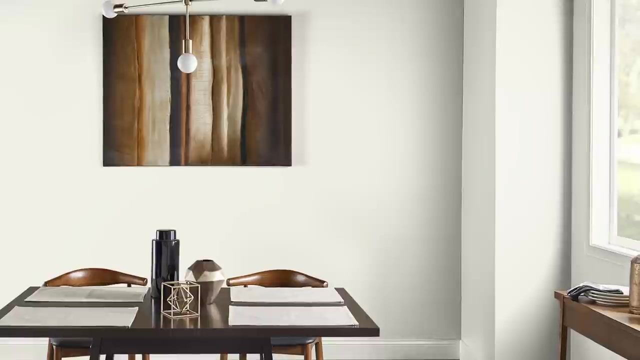 ceiling. you can always just leave them as they are because most likely it'll be a stark white up there, And then you just paint all the rest of your walls West Highland White- Totally a good option. Next up, we have one of the most immensely popular off-whites, not just in the Sherwin-Williams catalog but in decorating in. 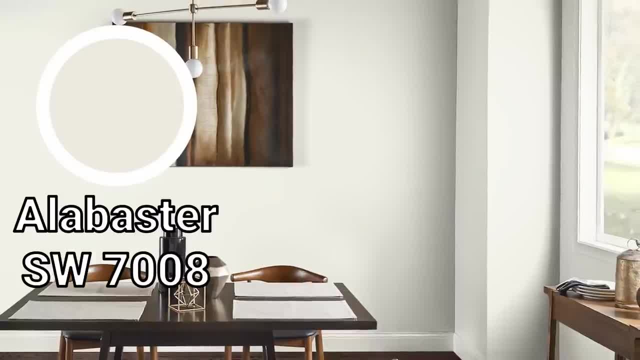 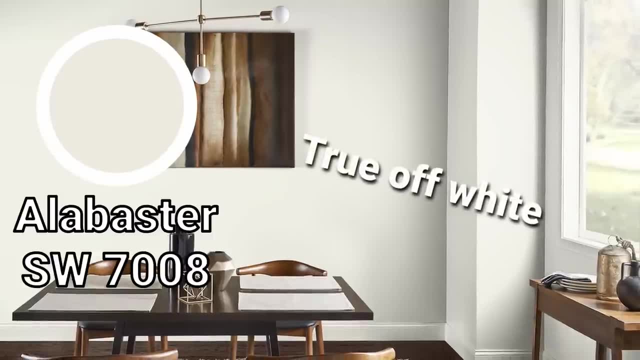 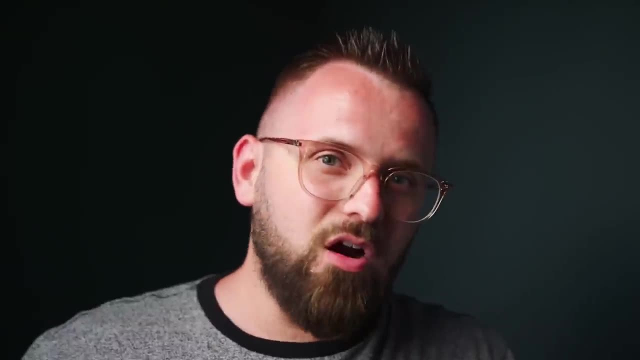 general It's Alabaster, which is an incredibly versatile, satisfying to use paint color that is perhaps on the borderline of feeling like a true off-white because of its LRV or its lightness score- you could say It's 82, and that makes it a bit darker than West Highland White. 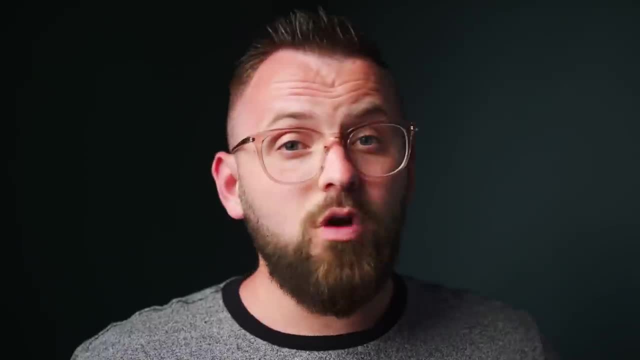 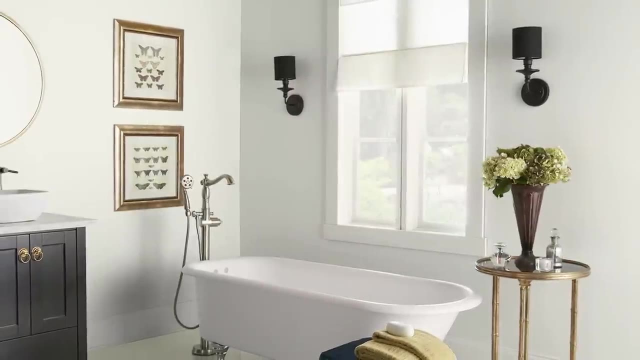 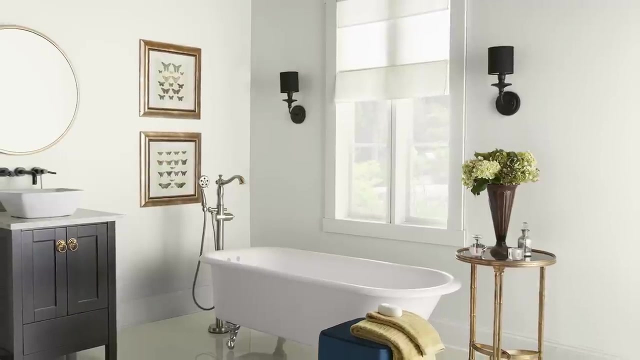 It also feels a little less creamy because its warmth is not so much from yellow but more so towards a toned down gray beige coloration. This makes it a powerful design tool because, whether you like anything remotely beige or gray related, it will more than likely connect with whatever palette you fancy. 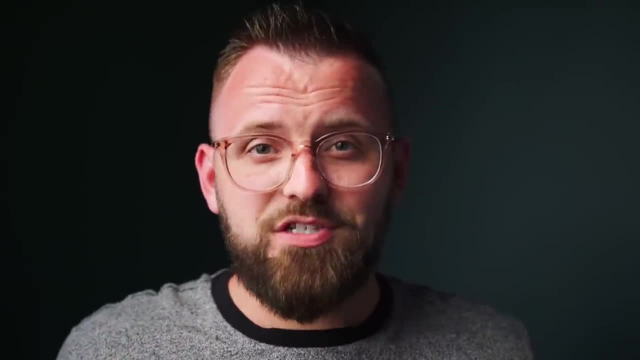 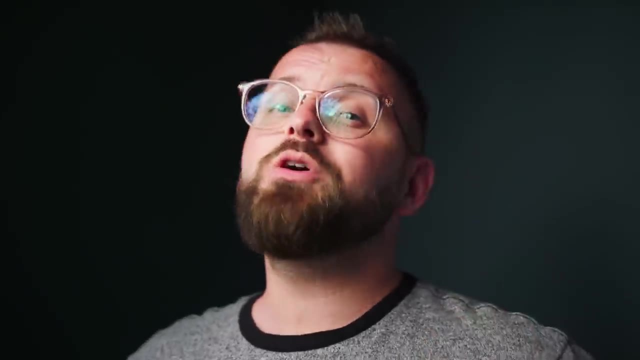 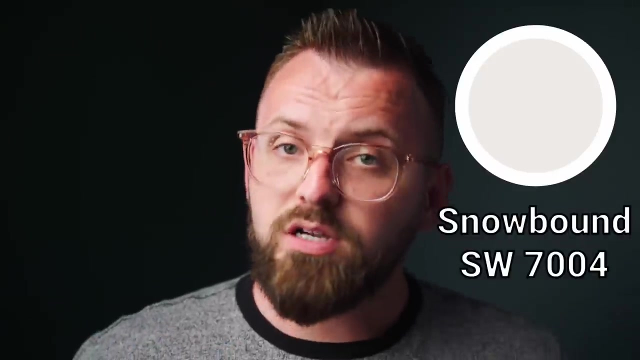 This next color is for the people that maybe don't have a ton of beige that they want to incorporate, but still need an off-white that is soft, neutral and timeless. That color would be Snowbound, which I think is a distant cousin of Alabaster, due to the fact that they're both technically warmer colors. 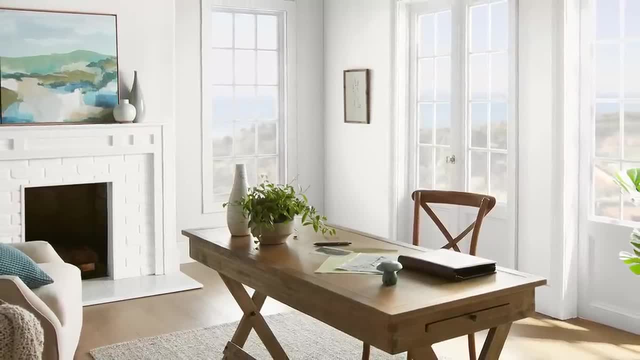 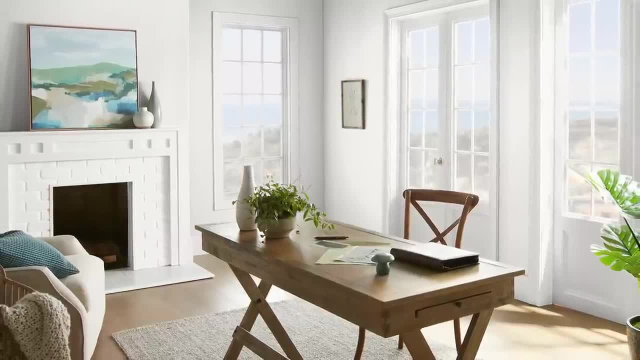 and that just means it reflects 83% of the color. and that just means it reflects 83% of the color. Snowbound's warmth comes a little bit more from Taupe, a combination of gray and brown rather than beige. Snowbound's warmth comes a little bit more from Taupe, a combination of gray and brown rather than beige. 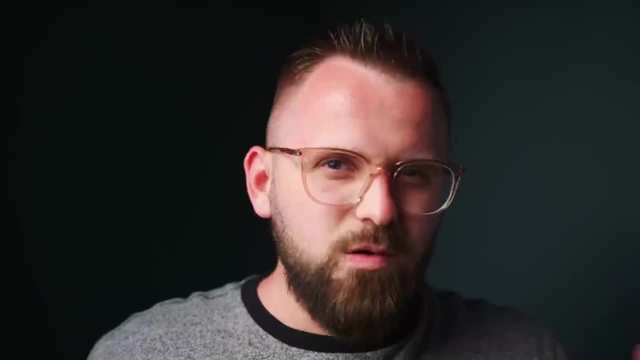 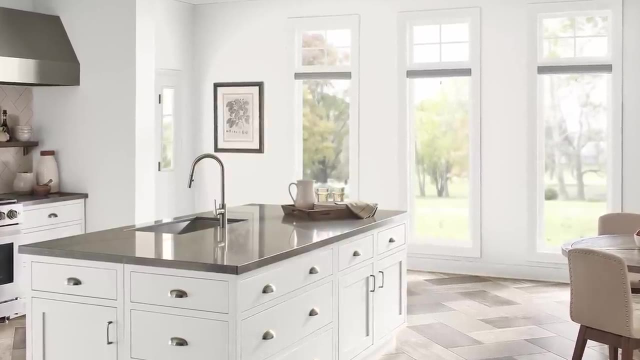 When brown is mixed into neutrals like this, you could also equate it to a very slight red undertone, but that would be misleading because you wouldn't really see any red in a color like this. Basically, if you like brown, but you want an offwhite all over the walls in your home, 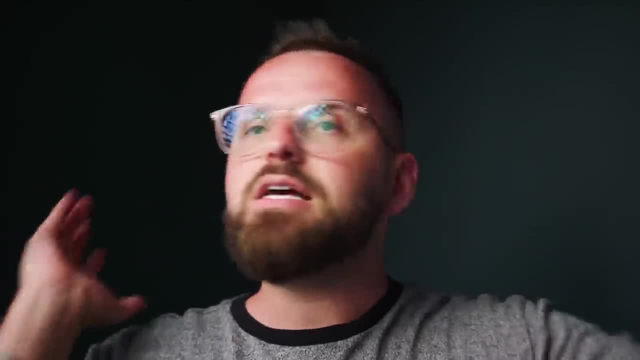 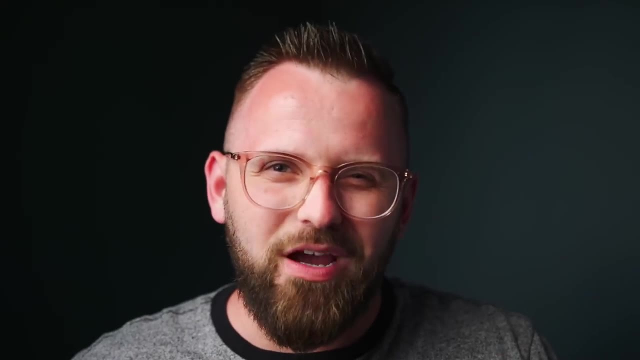 this might be a good one to start with. Now I know there are some of you that are just looking for a pure white And you don't want to heed my advice of playing with different undertones and different off-whites. Well for you. I'll just give you pure white, because that's what you asked. 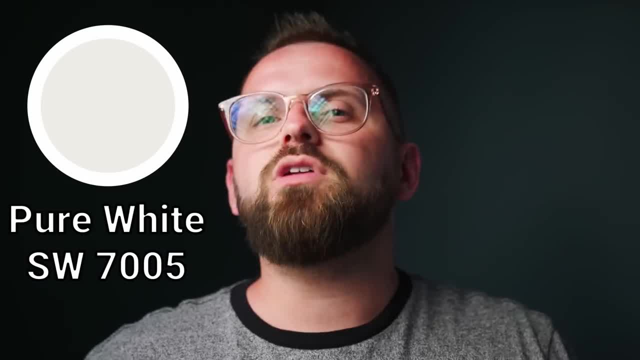 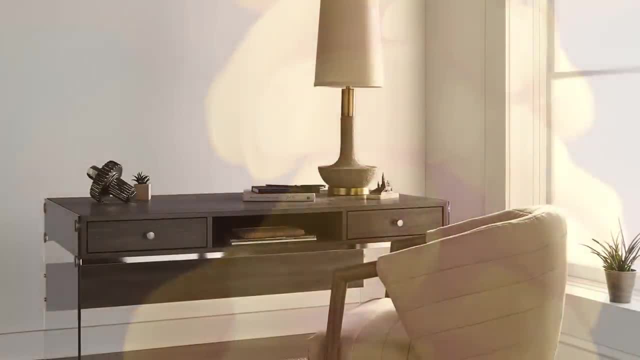 for It's pure white in the sense that it doesn't feel overly yellow or creamy or, on the other hand, blue and cool. It's pretty much right in the middle and it's very soft, has a bit of gray, so it's not overly bright, which is why it makes for a good candidate as a whole house color. 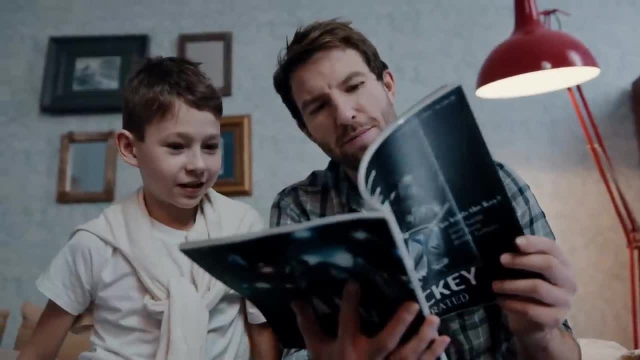 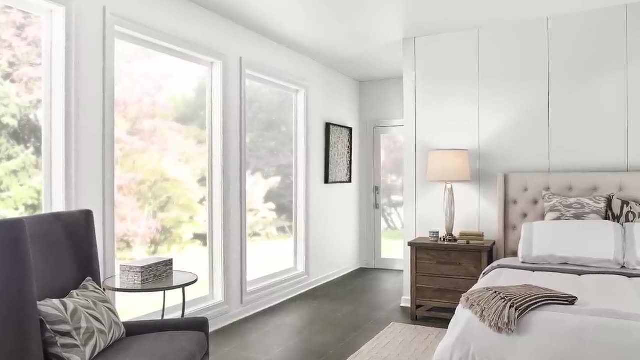 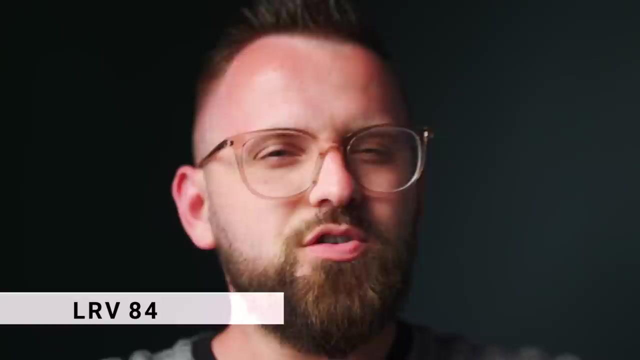 It may not be the most interesting choice, but for the epitome of a clean slate color, I think you can't really go wrong with pure white. It has that dash of gray and the slightest tint of yellow to keep it settled. and it's 84 LRV means it's bright, but not to an aggressive degree. So 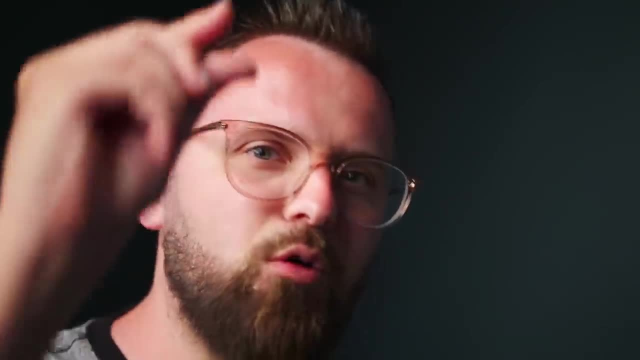 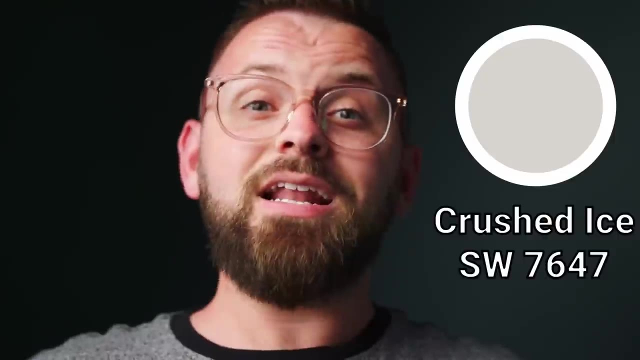 now that we got the off-whites out of the way, it's time for a little bit more color, or at least depth. I also want to cool things down a little bit with a color called Crushed Ice. Coincidentally, this color isn't. 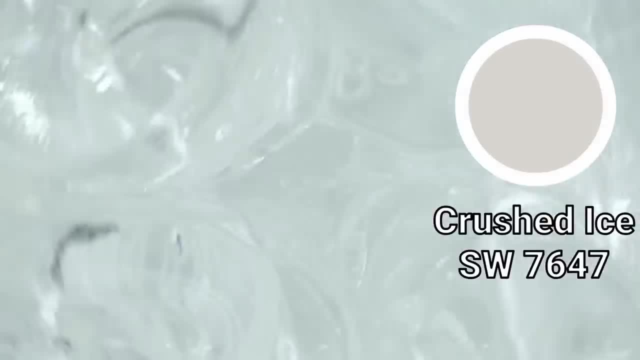 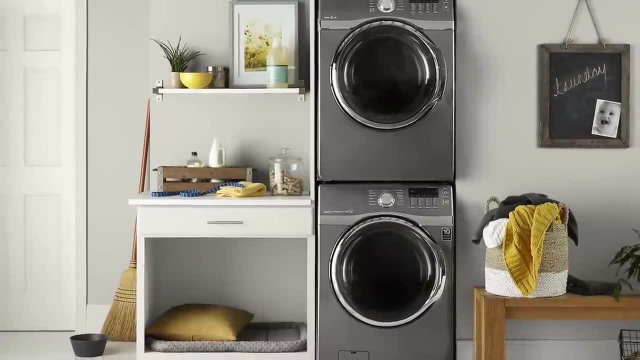 actually quite as icy as its name suggests, and I always see it as a light, warm taupe that is obviously under-saturated and gray-leaning. It looks like gray that has had a little bit of warm brown mixed in to eliminate any blue coloration, Although I wouldn't call it a cool color on its. 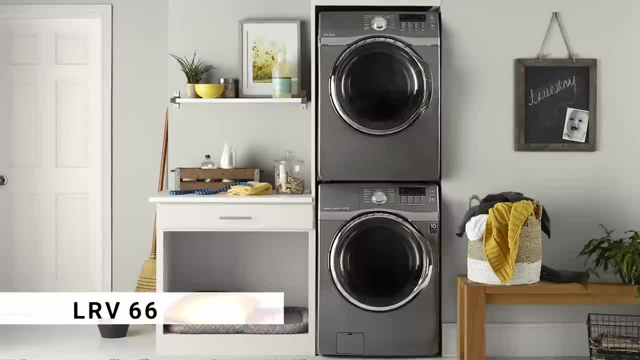 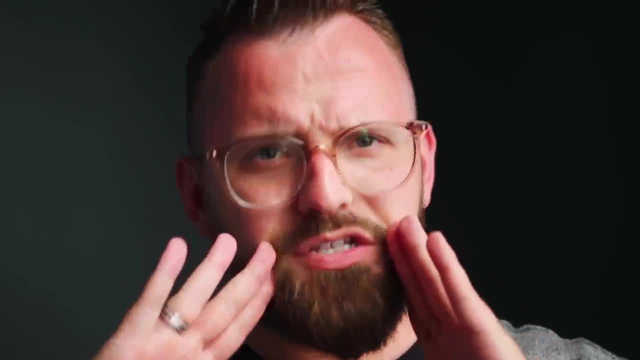 own. it can be a pretty nice transitional neutral that can help connect the dots between frosty grays and cozy beiges. You may be thinking, James, why do I need a transition color if I'm only picking one color for my house? I don't know. I'm just going to pick one color for my house. 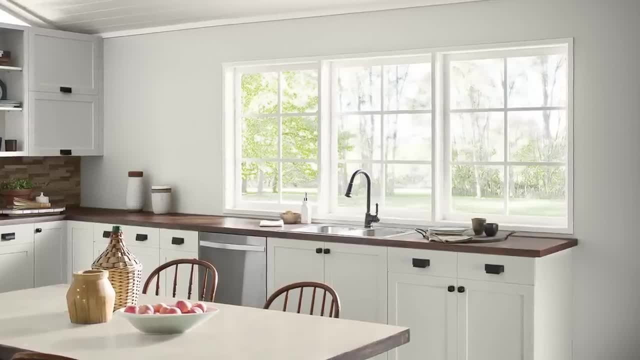 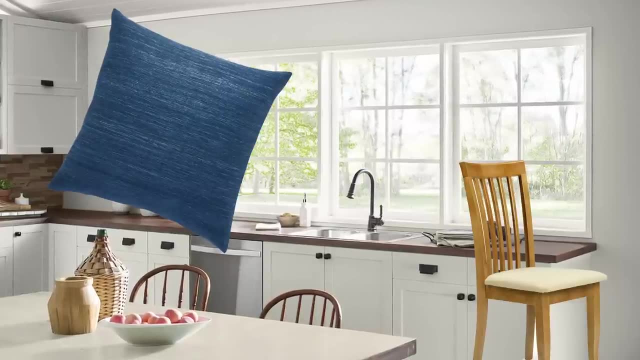 Well, you also need to think about the other elements in your home, like your flooring, for one, But more importantly, everything that's in your home, like your furniture, accessories, airy rugs, all that. Maybe you have a pretty contemporary kitchen and dining area that's. 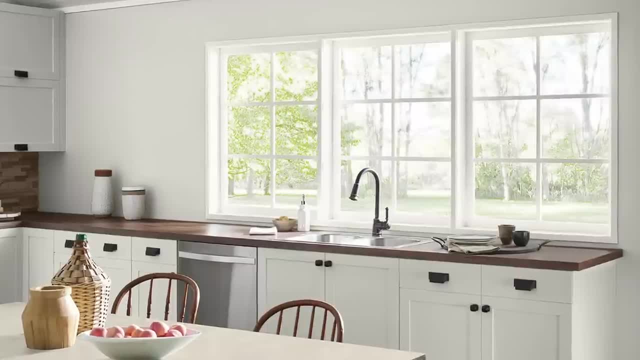 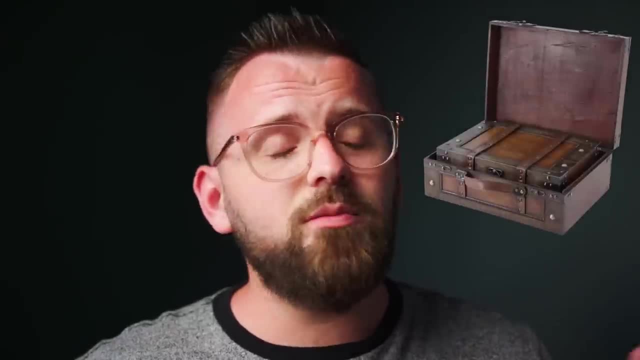 modern and contemporary and has a lot of cooler grays. but then you have a family room that is much more warm and cozy and maybe contains some beautiful antiques passed down from your grandmother. So that's where a color like Crushed Ice could incorporate itself in a 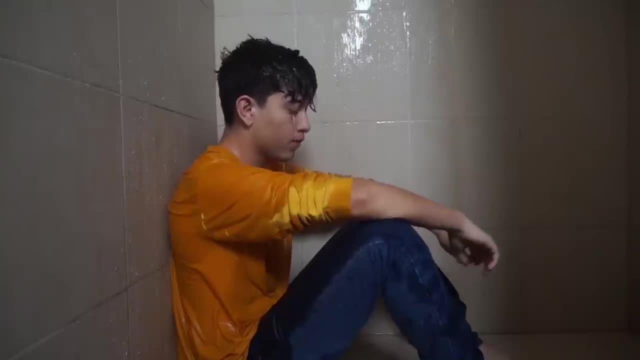 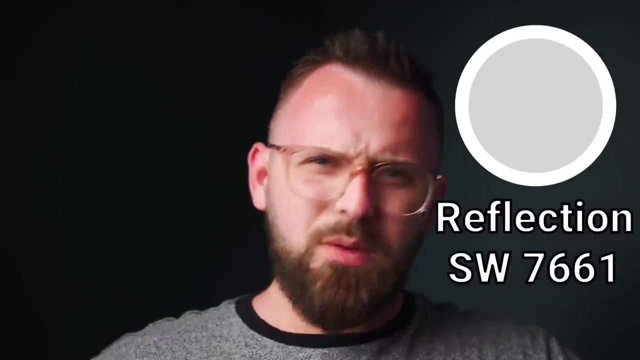 room in either of those spaces, And that's a plus. If you were a bit bummed out that Crushed Ice wasn't very icy, then maybe you'll be more interested in reflection, which is technically a pretty balanced gray with RGB values that are almost identical. Very quick side note. 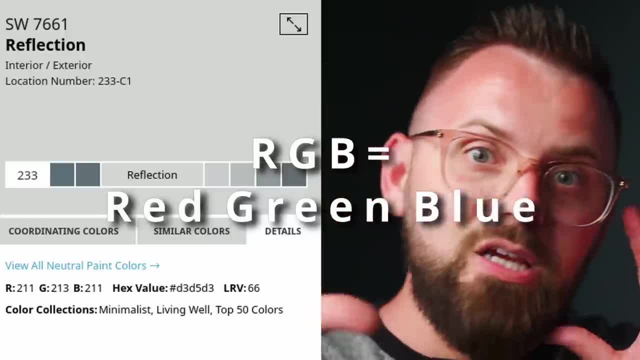 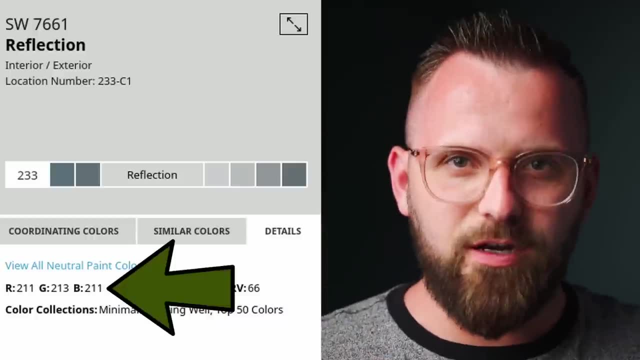 RGB stands for red, green, blue, which is just a way to digitally represent the ratio of colors found in reflection, And they're all pretty equal, with green just being a tiny bit higher. Also, subscribe if you want to catch a more detailed video. 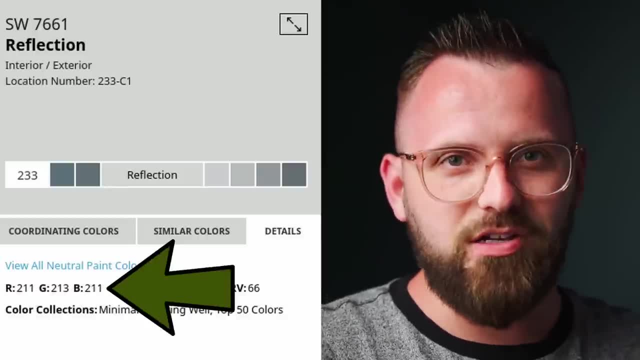 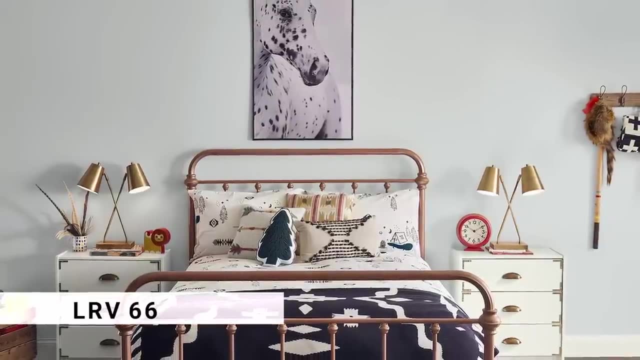 of what the heck RGB values are all about in regards to paint colors, because it's a little confusing. That video is in the pipeline. In actuality, reflection brings forth a pretty noticeable blue undertone, even though it is fairly balanced and muted. I've seen many people use this color throughout their 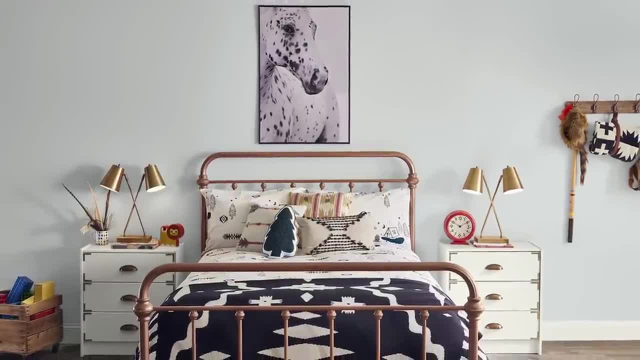 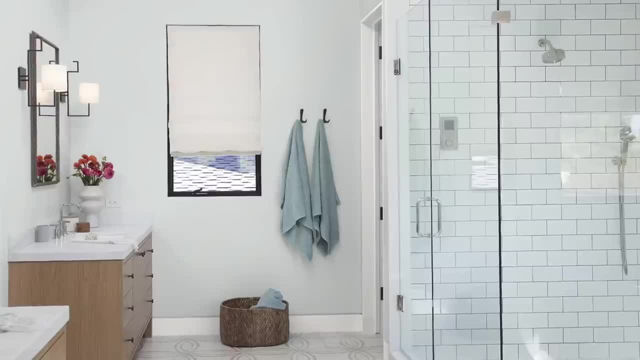 home, and even though it's not a traditional looking color, it could really suit certain interior design styles pretty well, more so on the transitional or modern side, or even coastal. This is especially the case when you incorporate it next to a really crisp, stark white trim color. 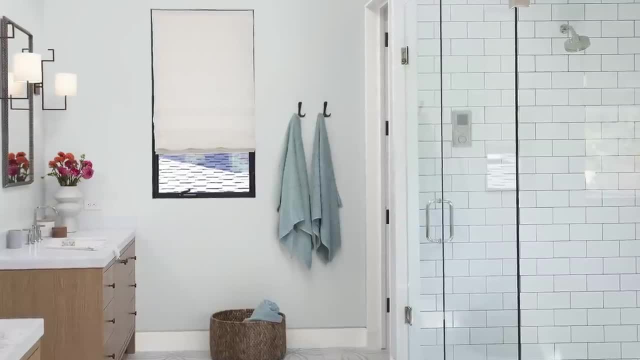 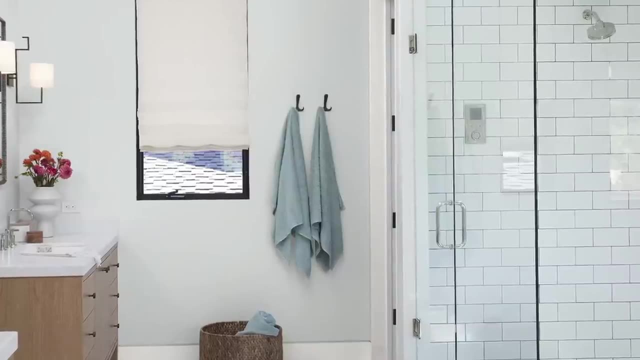 to cut through like a high reflective white. So these last two colors are just as dark as one another with a 66 LRV. but for this next one we get a little bit darker and a bit more green, which I'm a massive fan of. The color is called conservative gray and it's just a bit darker than reflection. 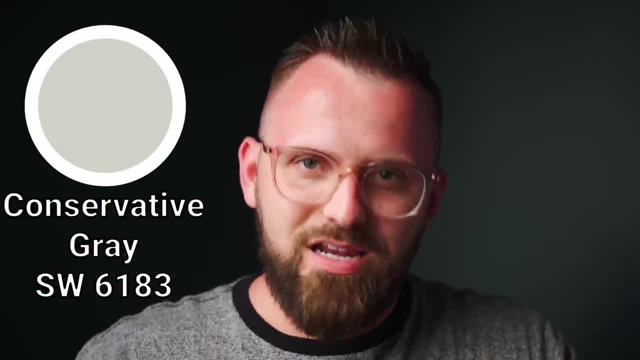 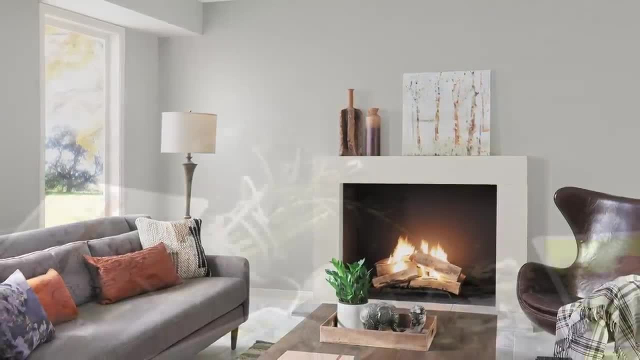 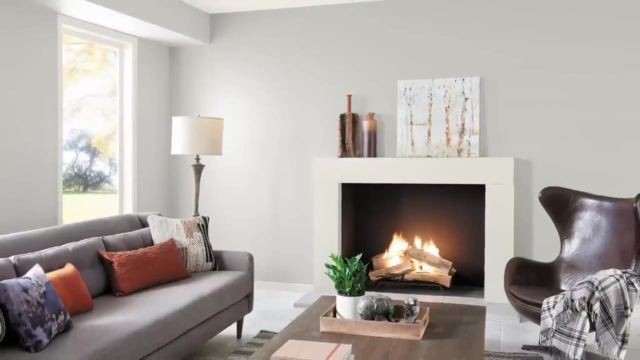 but it sort of evens itself out with that added warm green in the undertones. I'll be the first to admit that this is perhaps more of a trendy choice, because everybody's talking about sage green and those greeny, gray, beige colors which we could argue conservative, gray being one of those. 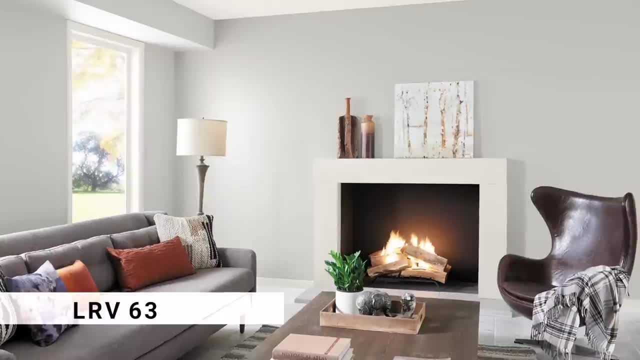 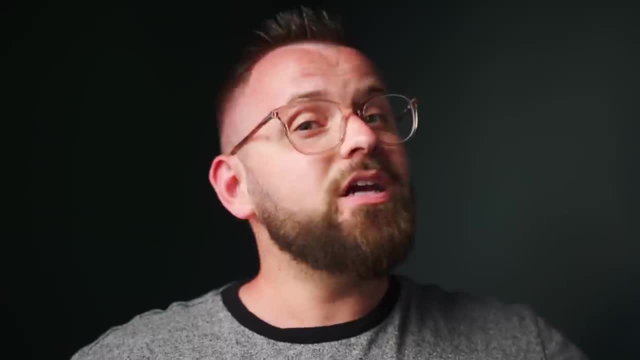 things, But I am hoping that this is a trend that'll stick around for a while, because it's just an interesting alternative to traditionally beige leaning neutrals on the walls. Green also loves more green, So if you're someone that loves to incorporate plant life greenery. 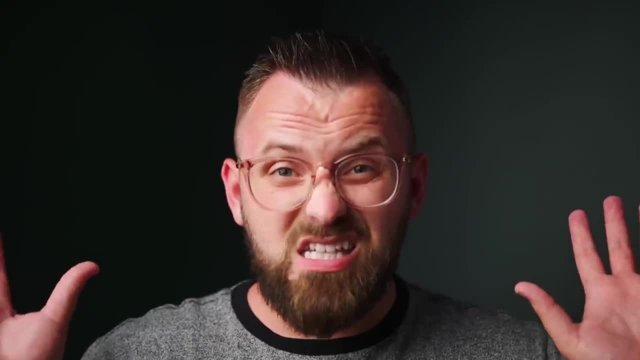 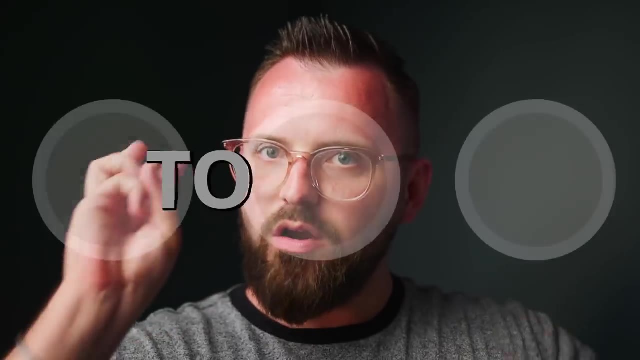 and even fresh flowers in your home, maybe a bunch of succulents everywhere. don't water them too much, then conservative gray will really come to life in those types of environments. That being said, there are three Sherwin-Williams colors that are pretty much the top tier of. 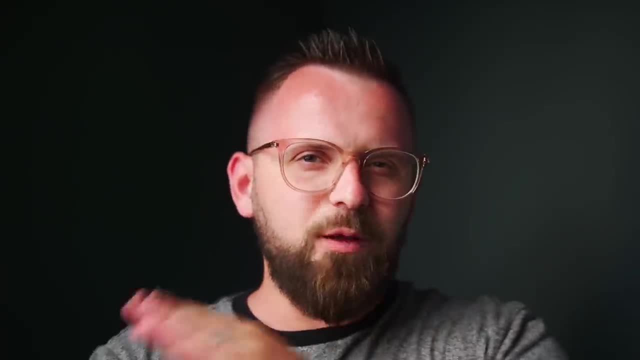 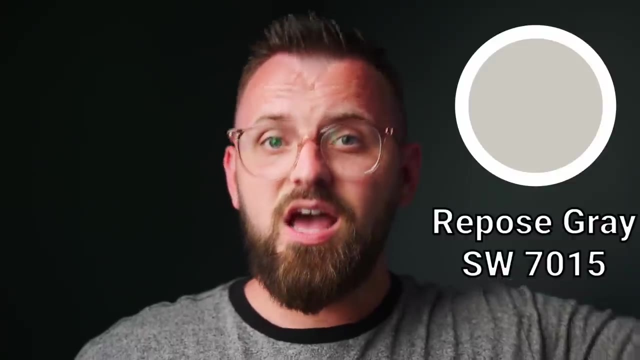 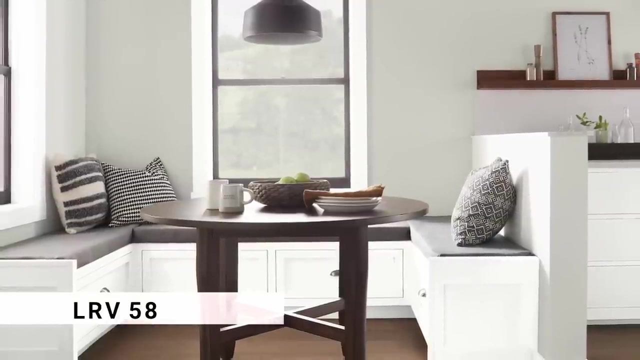 whole house paint colors. We'll start cool and slowly get warmer and warmer with each one. The first one is repose gray. Tied for the darkest color on this list. repose gray is probably the coldest, mega versatile paint color that exists. It has that slightest tint of warmth. 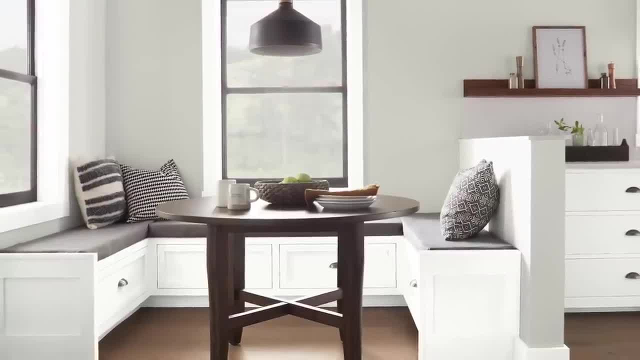 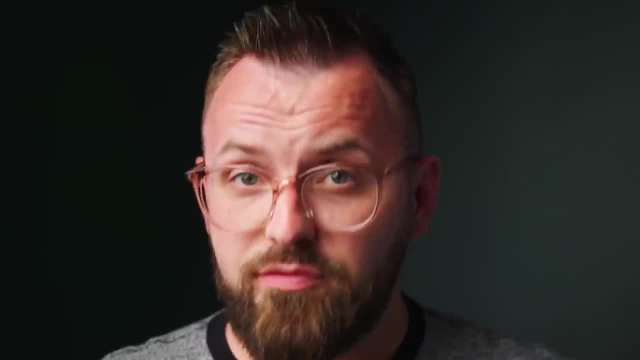 in the form of a dash of brown, but it's a large amount of gray that takes precedence here, almost to the point where it sometimes has a subconscious green undertone, not nearly as much as conservative gray, but it's still present. I still like to. 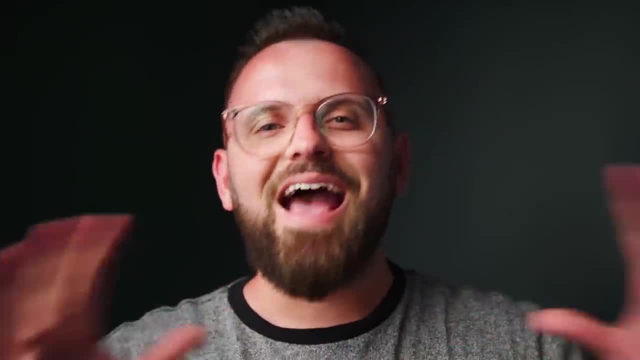 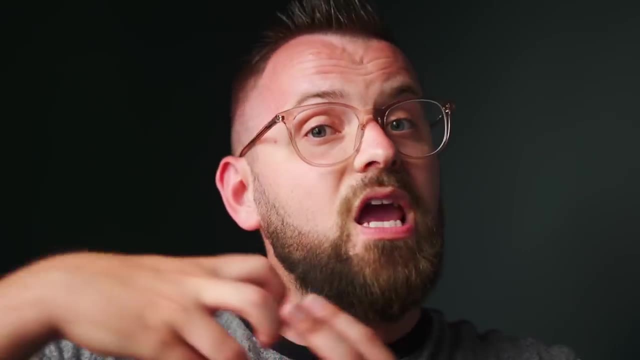 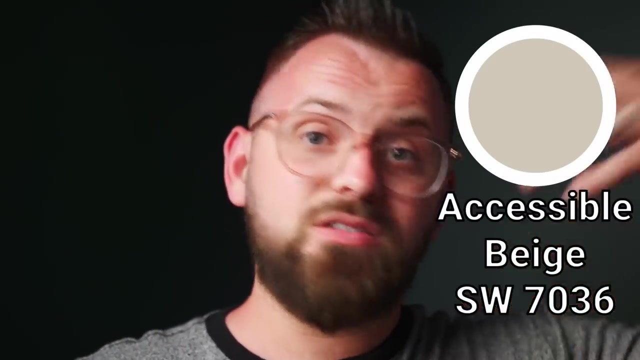 define it as a topi gray, which is fantastic for those more modern homes that are looking for something solid and stable. If we flip the script a little bit and lean way more into beige, but stick around that same LRV, you have accessible beige, which is just as dark as repose gray.